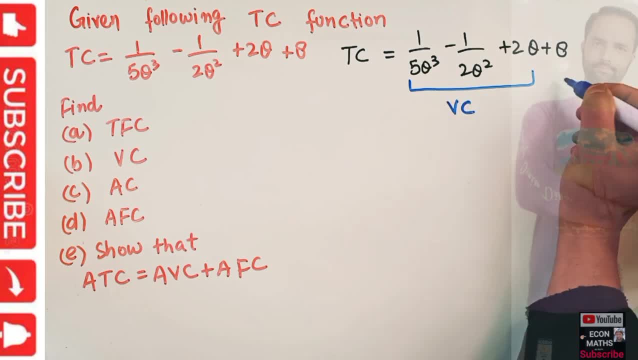 denote our variable cost and this last term denote the fixed cost. Why? Because total cost will change with the change in output. here because q is in each of the first three terms and fixed cost is 8.. It does not depend upon the level of output, Whether the output is 0 or anything. fixed cost: 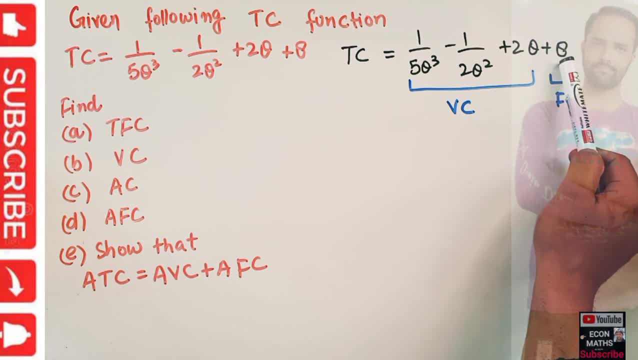 will remain same. That means this fixed cost, which is 8. here it does not depend upon the level of output, okay, But the first three terms actually depend upon the q. okay, Last term does not depend upon the q, That means it is the fixed cost and first three terms are the variable cost, because 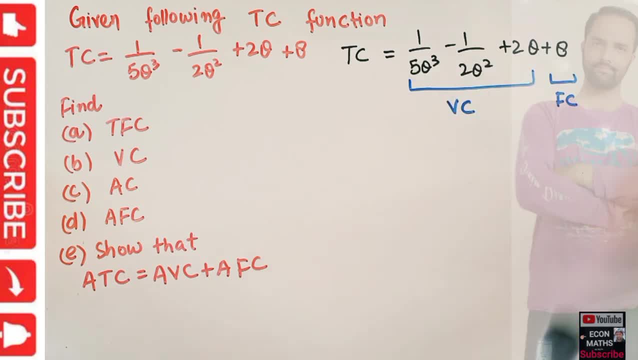 they change, Total cost is 8.. The variable cost will change with the change in the output. okay, So first three terms are variable cost and last term is fixed cost. Let's write it here. That means our variable cost is equal to 1 upon 5 q cube minus 1 upon 2 q square plus 2 q. This is our variable cost, Fixed cost. 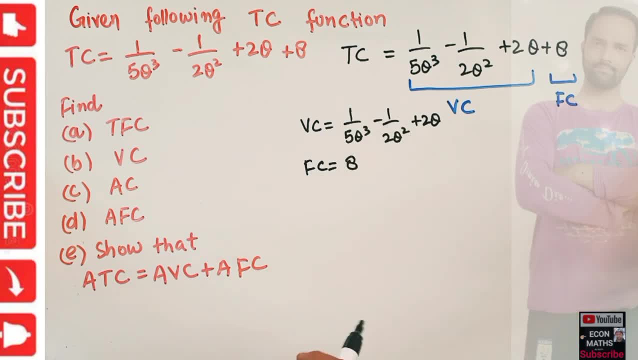 is simply our 8,. okay, This does not depend upon the level of output. First thing we need to find, we need to find out the total fixed cost. So our total fixed cost, or fixed cost, is equal to 8.. So 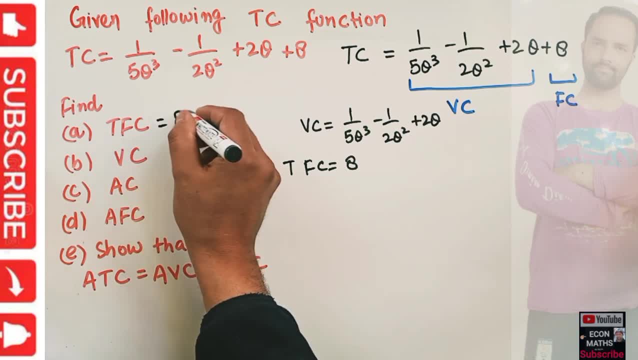 this is, our total fixed cost will be equal to 8 and our variable cost, as we have calculated it, came out to be 1 upon 5 q, cube minus 1 upon 2 q, square plus 2 q, because this depends upon the level of output. Third part is to find out the average cost. okay, Average cost when we are being told it. 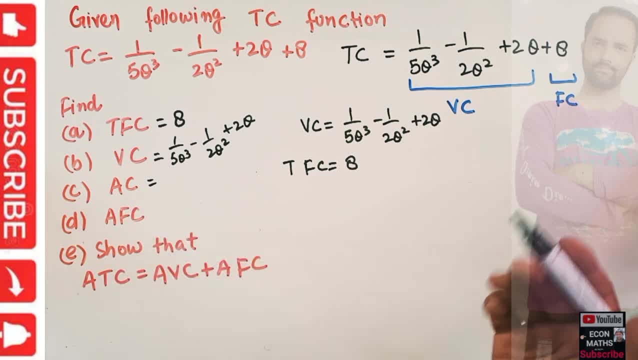 means the total cost upon output. okay, So average cost. if I write it here, Average cost means our total cost divided by output. Total cost function is this: That is, 1 upon 5 q cube minus 1 upon 2 q. 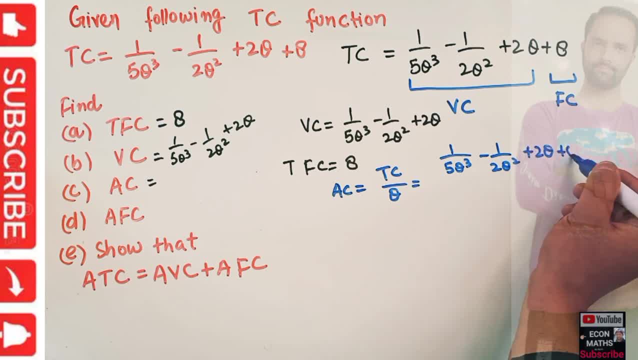 square plus 2, q plus 8.. To this we divide by the output: q. okay, Which implies it is if we divide q to each of these terms. So first term will become 1 upon 5, q raise power, 4 minus. second term will become 2 q cube, okay, Simple division. Here it will become 2 q upon q. 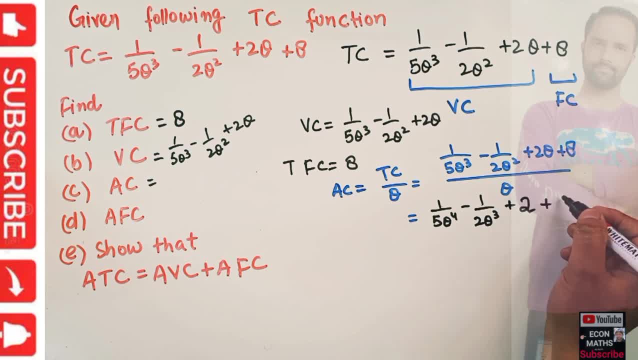 it will become 2 plus 8 upon q will be 8 upon q. okay, This is our average cost. So this denotes our average cost, which is 1 upon 5 Q raised power 4 minus 1 upon 2 Q. cube plus 2 plus 8 upon Q. now last is: 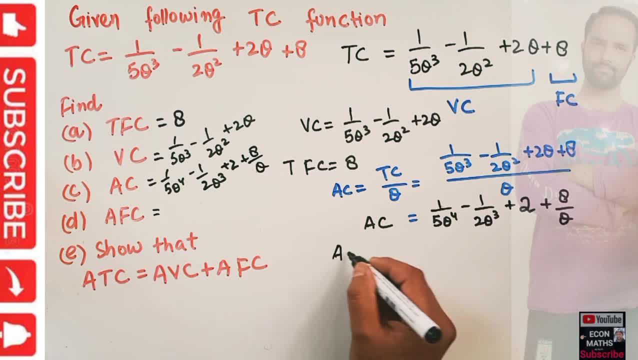 average- sorry, D part is average fixed cost. average fixed cost will be equal to our total fixed cost upon output. okay, so total fixed cost is 8 to this. we divide by output, this becomes our average fixed cost. so it is 8 upon Q. last is show that average total cost is equal to average variable cost plus. 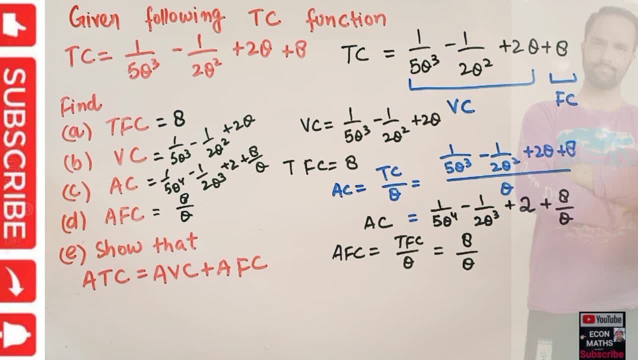 average fixed cost. for that we need to calculate the average variable cost first. okay, this is our average cost here. so our average variable cost will be equal to the variable cost upon output. okay, so variable cost is this function: 1 upon 5 Q cube minus 1 upon 2 Q squared. 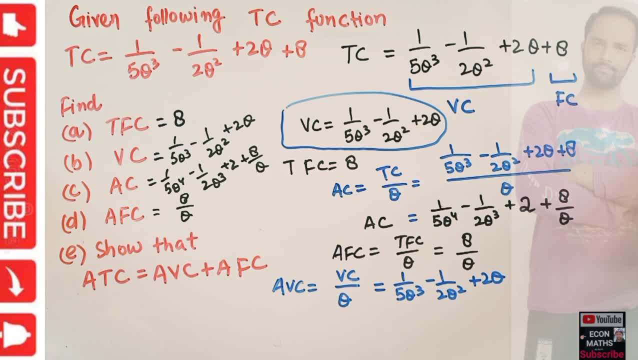 plus 2 Q. okay, this is our average variable cost. to this we divide by the output. so, dividing each term with Q, first term will become 1 upon 5 Q raised power 4. second term will become 1 upon 2 Q cube and third term will become only 2 Q. 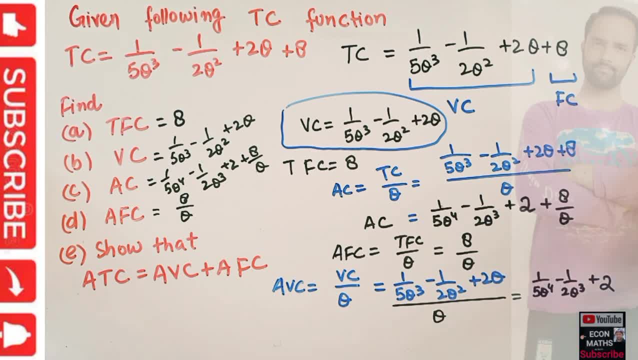 upon Q is 2. okay, this denotes our average variable cost. now, what is our average total cost? okay, so we need to calculate the average total cost also. so AC, it is all actually our average total cost. okay, or in place of AC, we can write average total cost, average total cost, so our average total cost. you can see our.